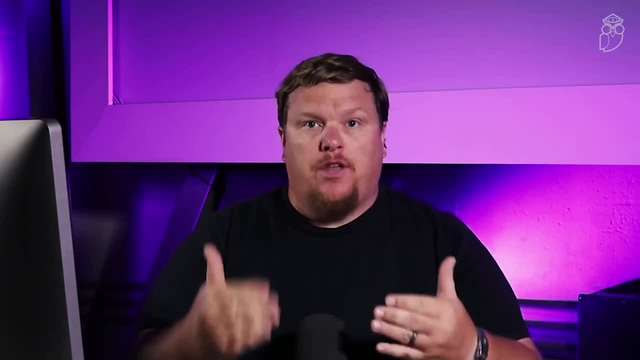 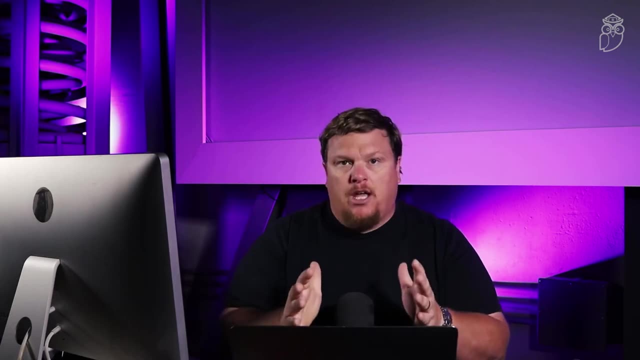 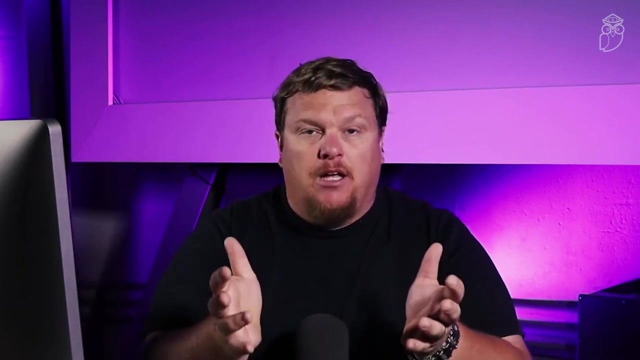 they're actually not very smart. They only understand two things: on and off. They can see light on, light off. Whatever it may be, it's only two things. In order for communication to happen, there must be some sort of a change in something. 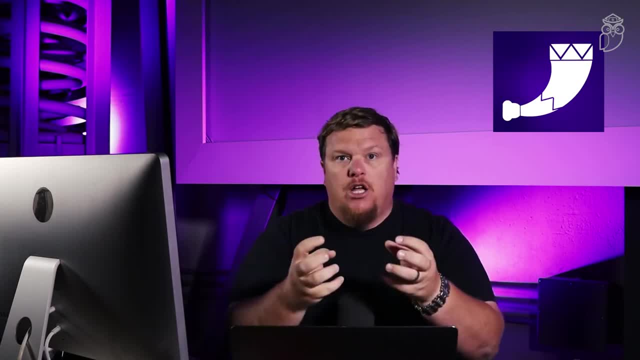 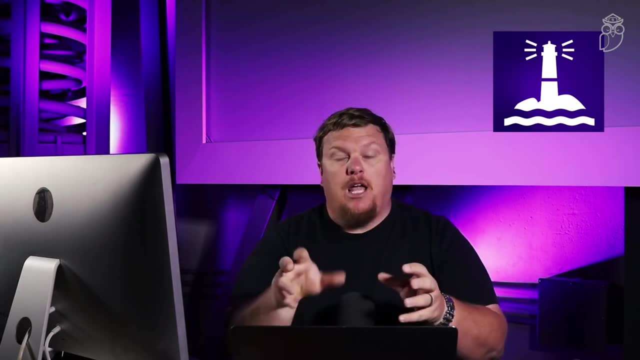 My voice is changing. It's getting louder and softer, in different tones. If I wanted to flash a light in Morse code, like if I had a mirror here, I could actually flash a light and I could communicate. You see the light and then you. 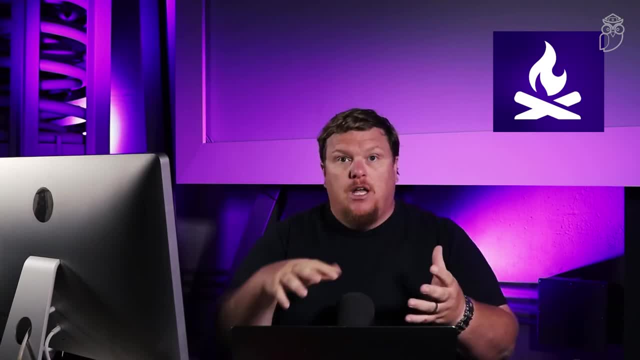 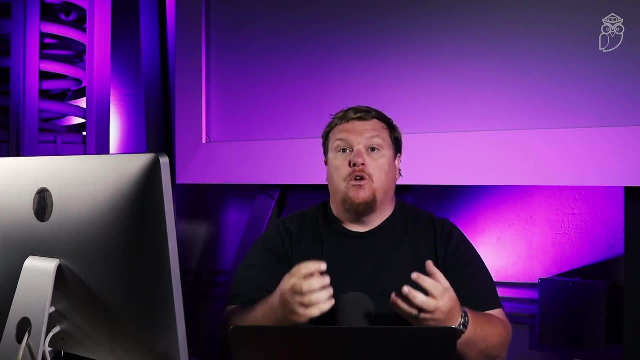 don't. You see the light and then you don't. Or think of smoke signals. So smoke, I see a ball of smoke and then nothing. A ball of smoke and nothing. There has to be change in order for any kind of communication. 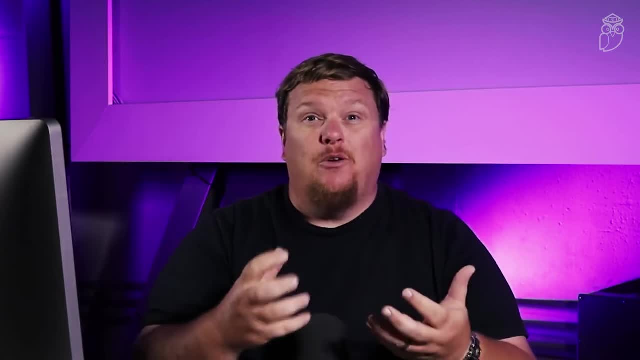 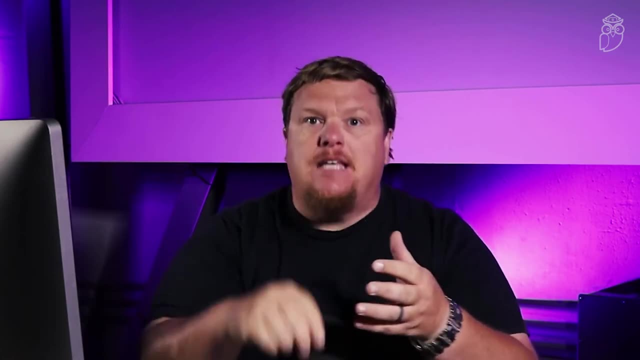 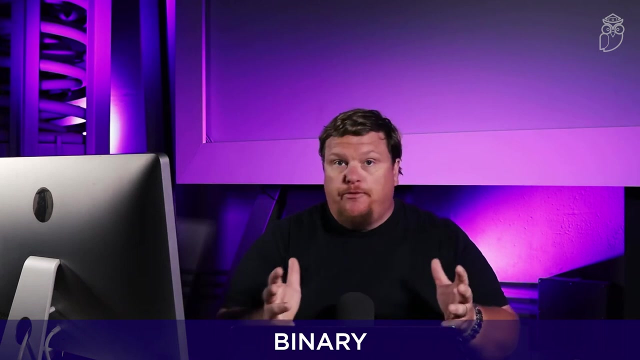 to take place. So in computing there's really only two states of something, just two ways. anything is at the most basic level inside of any computing device, So that is called binary. So we have these things that you've heard before called bits and bytes. So a bit is very simply. 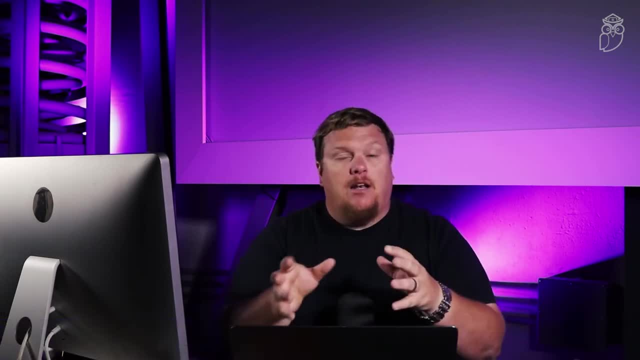 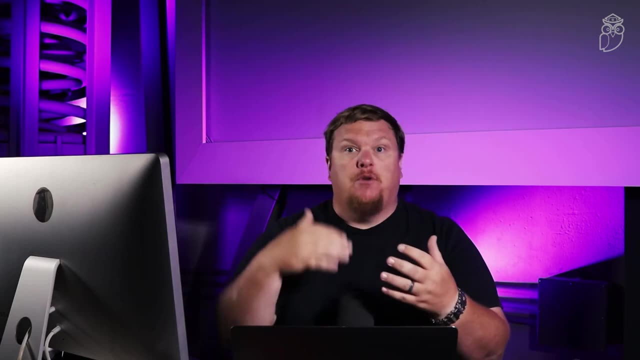 a zero Or a one. We're going to talk about this again in another video. We learn or we have this, this base 10.. We know the numbers zero through nine Computers. they know those numbers but, again, at their basic level they only understand zeros and ones. That's called base. 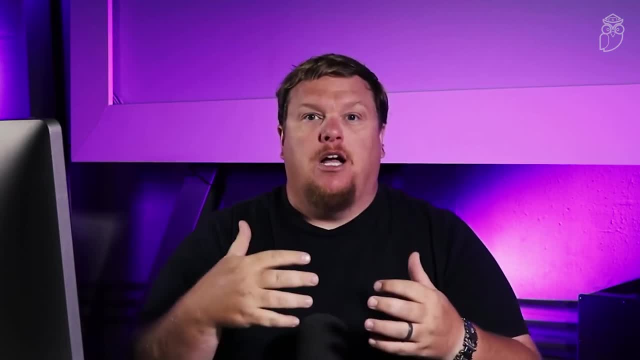 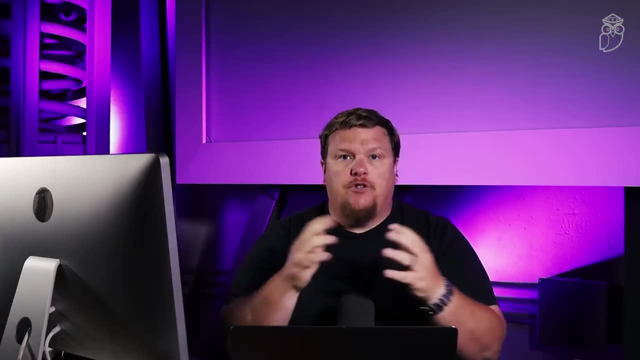 two. We're in a base 10 society because we have 10 fingers. Computers only understand two things: zeros and ones. So it is what's called base two. So let's put this in real life terms for you. So something- hopefully that is something you've encountered before- When you download a. 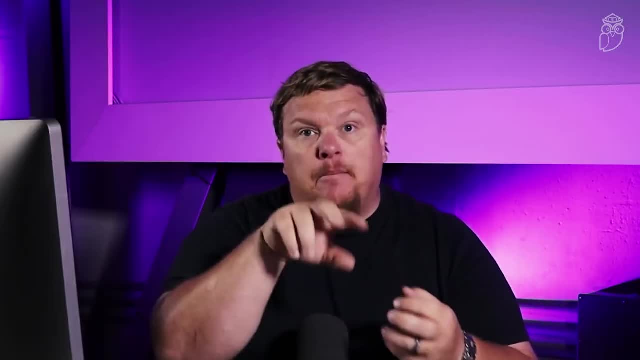 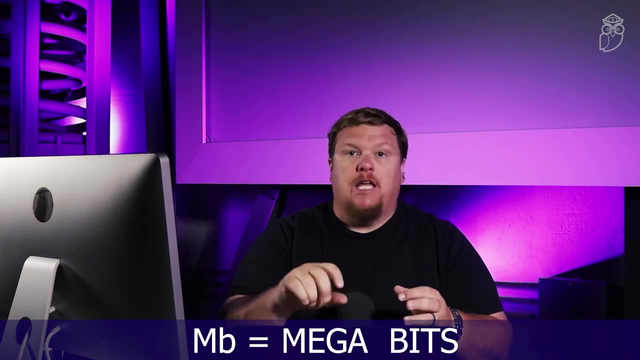 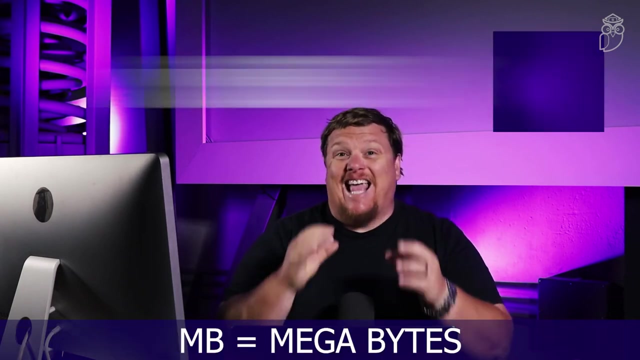 file. maybe it will say: oh, this many MB megabytes. or M little b megabits. So the B, a lowercase B is bits. That is again a singular one or a singular zero. A byte is eight of those. 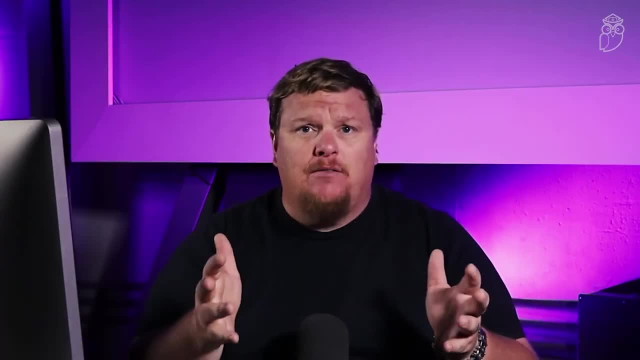 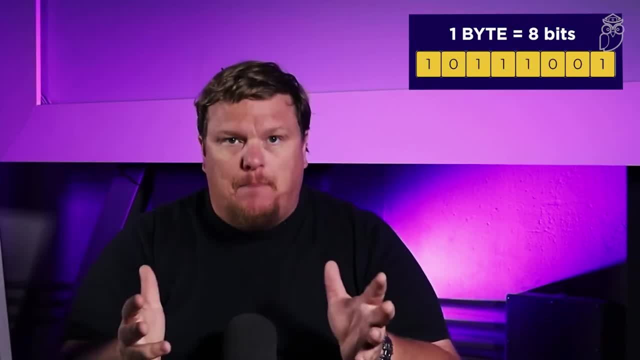 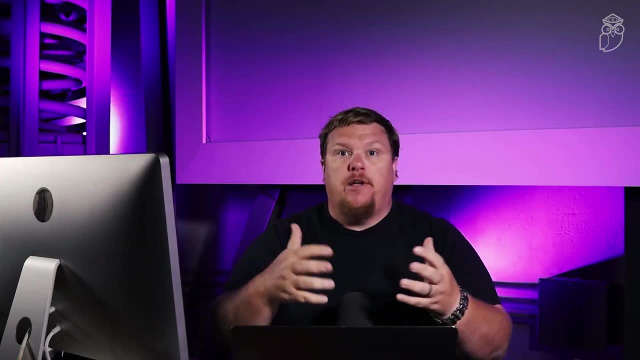 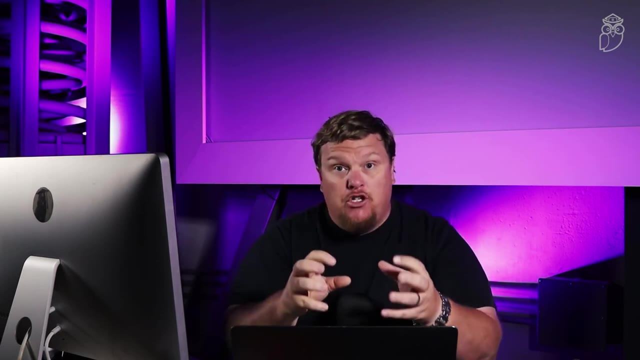 Hey, eight of these make sense to put together and it's called a bite. Now the bite is represented by a big B. Now, since old school days, like 50 years ago, 60 years ago, people would in computing, they would talk about bits and bytes individually. 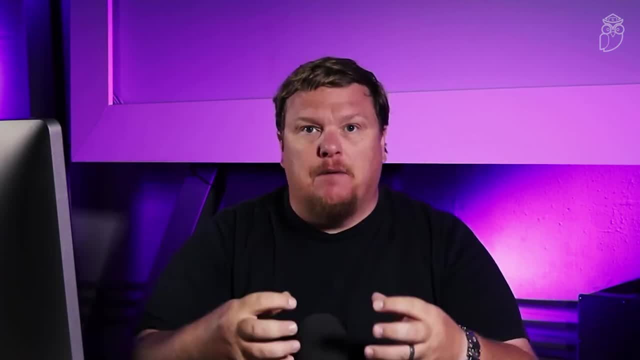 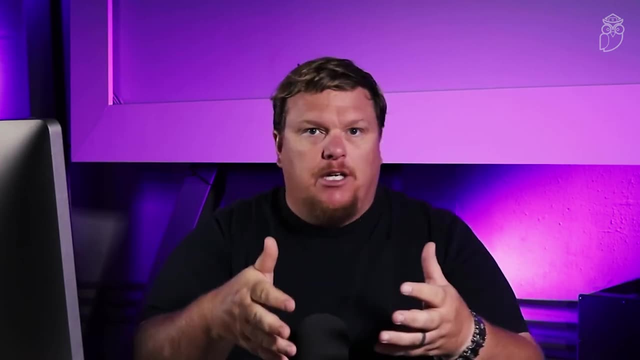 Now we talk about things like megabytes and gigabytes and terabytes or terabits, Those, the giga, the mega, giga, Tera. I might as well just tell you what that is: Megabits and Mega is million, so there's kilo, which is thousand. 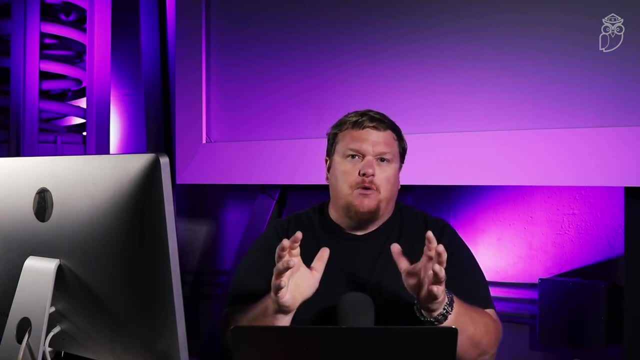 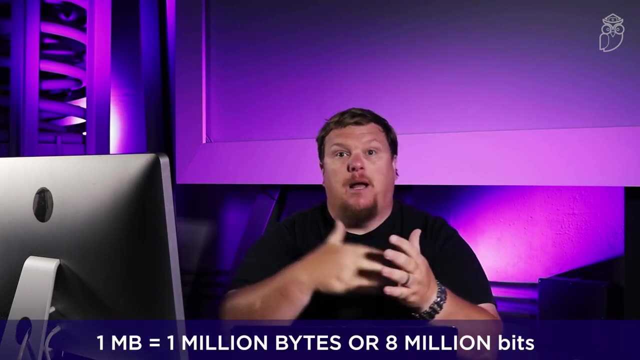 But just to throw more craziness in here, it's actually not a thousand, it's 1,024.. Again, we'll talk about that later. I know this is a confusing first video already, But just think this: kilobytes, megabytes, gigabytes. 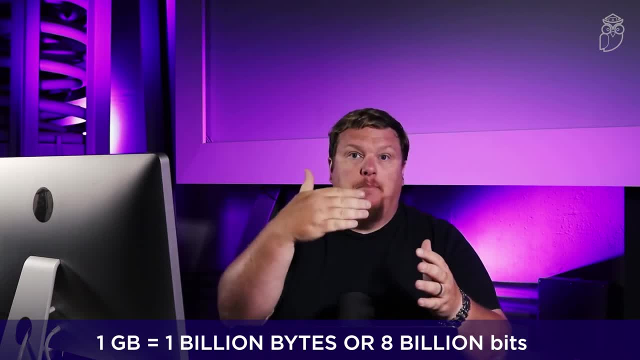 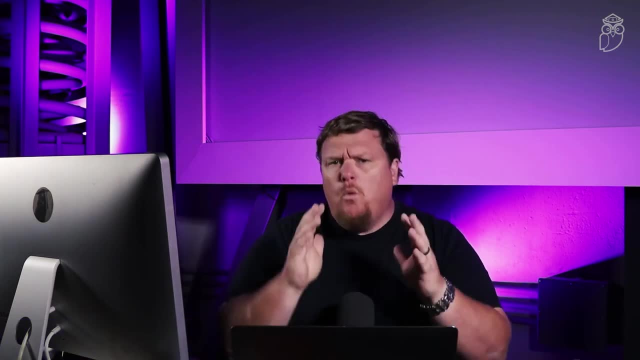 those are thousand, million, billion, terabytes, whatever comes after that. hundreds of billions, So big numbers of bits- One of the things that you know. leaving this video, what I want you to understand is that there has probably been some confusion in your life before on. 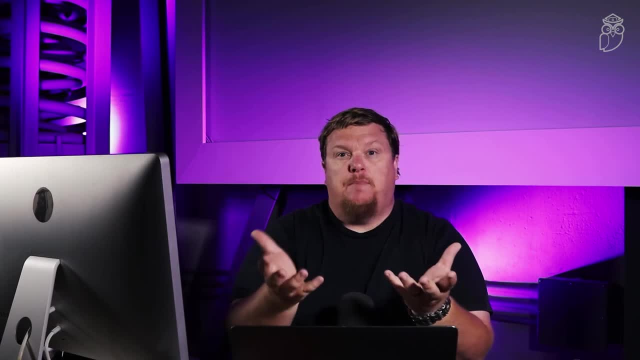 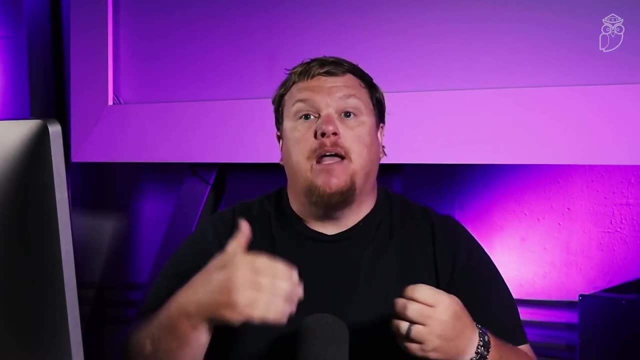 I'm paying for this amount of speed, but I'm not getting the speed on my internet that I expected. Well, one of the reasons is is that maybe you have a 10 megabit per second internet connection. Notice, I said megabit per second. 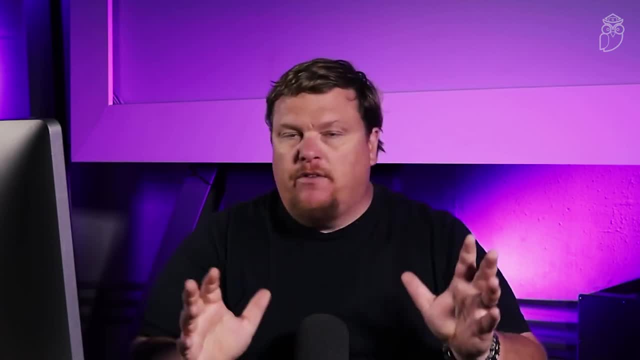 So that means I'm getting about 10 megabits per second internet connection. That's a million bits per second if everything is working perfectly Now, when you're using your machine- whether it's a Mac or Windows or Linux- to download. 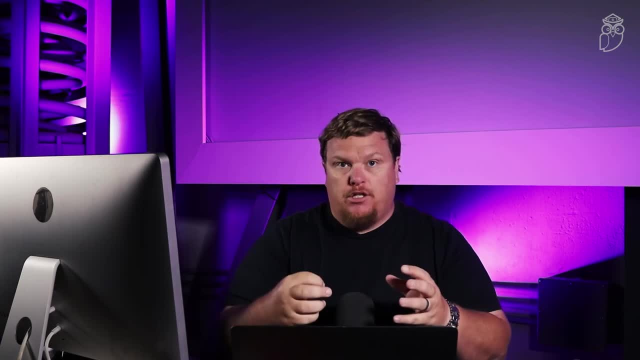 a lot of times they actually show you the transfer speed. So you're downloading your favorite song or videos or whatever it may be. It actually shows it downloading in megabytes per second. What's the difference between a bit and a byte? Eight X, eight times is the difference. 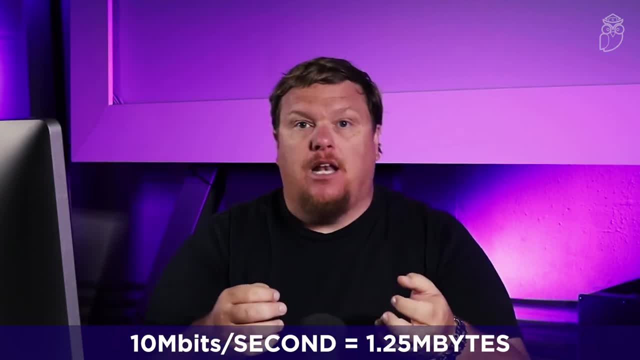 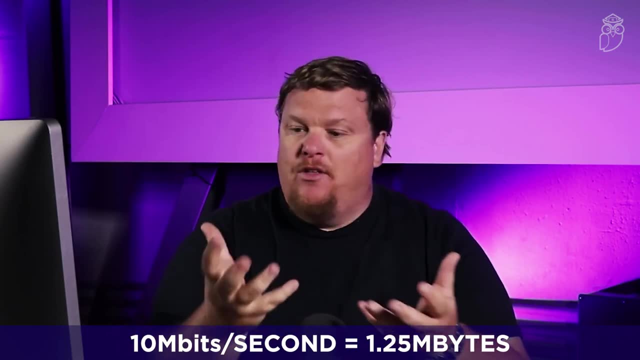 So while you're paying for that 10 megabit per second connection, your machine is showing something to you in how many megabytes per second it's downloading, and the numbers won't make any sense. They will look like it's really slow download.